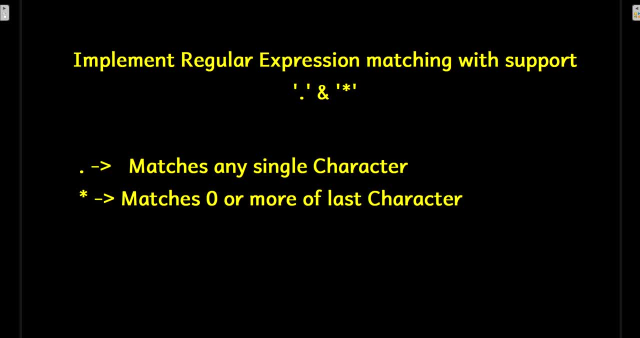 Hello, all welcome to Netset OS Today. in this video, we will discuss about how to implement regular expression matching with support of dot and asterisk. Coming to regular expression, we have more symbols to it: question mark plus and many more that we will discuss in the next video. 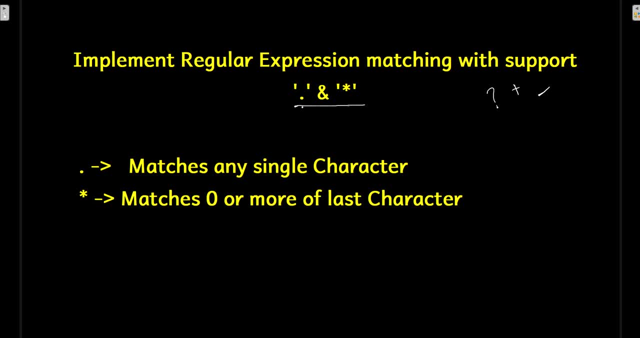 For this video we have dot and asterisk and we will know its complete implementation, starting from its basic going to advanced. So first of all, what it symbolizes. So here, dot means matches, any single character, Any single character. I mean to say, if I have a, dot b, we will have any single character to be filled. 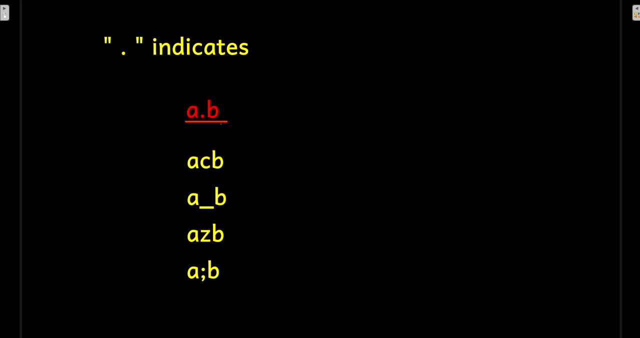 Within a and b. If I have a dot b, so this can be matched with acb a underscore b, azb a, semicolon b, So instead of dot we can have any alphabet, any symbol, anything but just a single character. 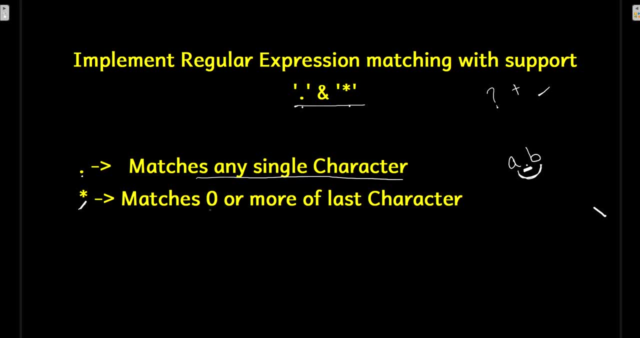 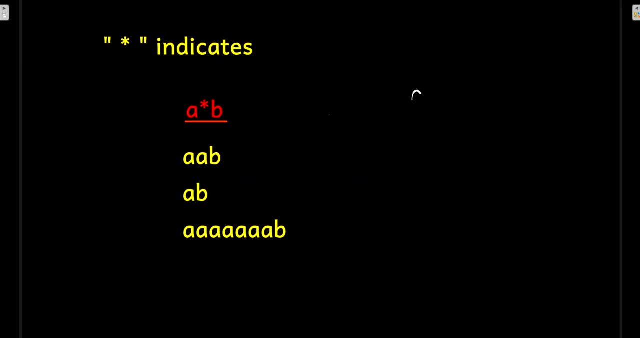 And if I come to asterisk, it says it can be matched With zero or more of last character. It symbolizes the occurrence of a Jiske ye peeche hoga. If I have a star b, that means it is going for its last character. 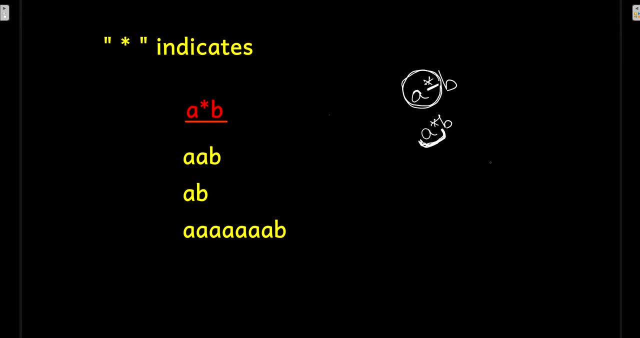 The occurrence of last character. The occurrence of last character can be from zero or more, But it should have a only. Let's say, if I look for a star b, I can have two a's together, Zero a together, Because a and b we already had. 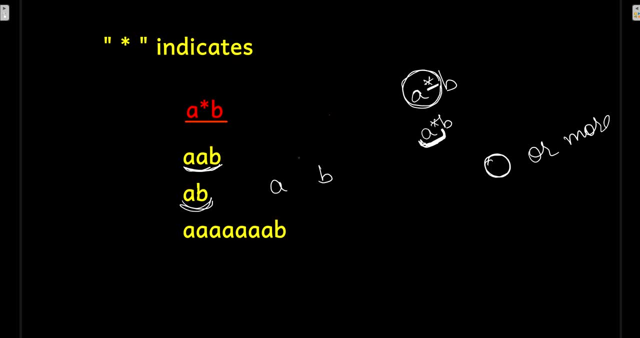 Instead of star. I haven't put anything. It is zero. The occurrence of a is zero over here. It will accept it, Or it can have various numbers of a. Let's look at practically. So looking into practically, we can go to. 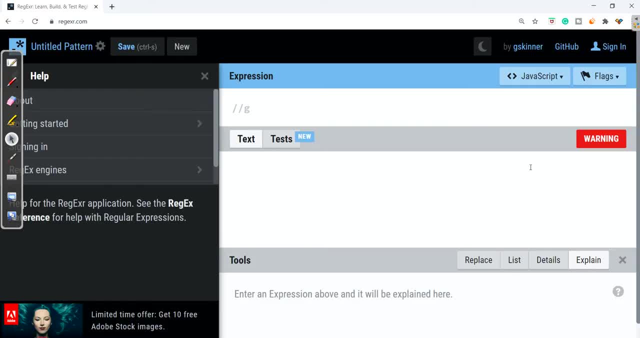 regexrcom. Here on this side, you can have a practical experience Where you can put an expression first. Let's say, if I write here ab, Here I need to give a text on which this expression should match with. Now, if I have here ab. 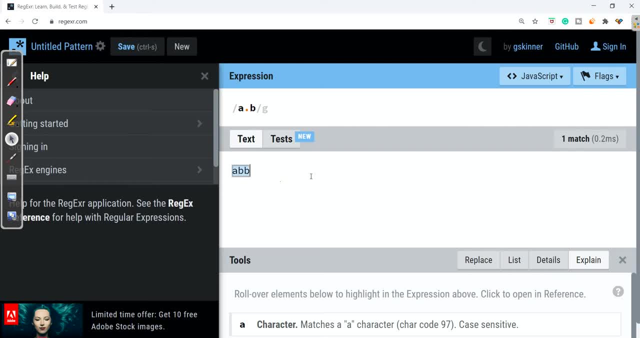 Dot means single character, So I can write a, b, b With this blue highlighting area. That means it is matching with ab. Now, here, if I write a underscore b, It is matching here. Here, if I write a, 2, b. 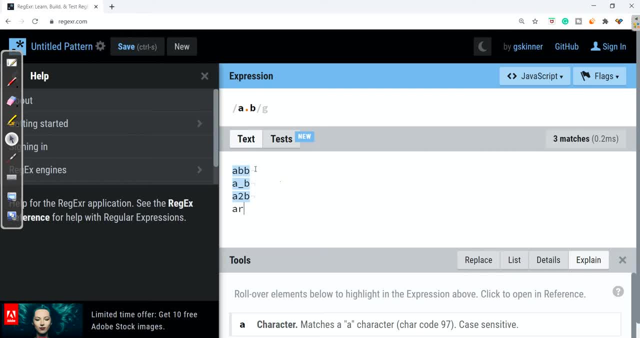 It is matching here. But if I write here a, r, t, b, Here it is not matching, Because dot always symbolizes its single character, Not more than that. But within this single character you can have anything. Now instead of a dot. 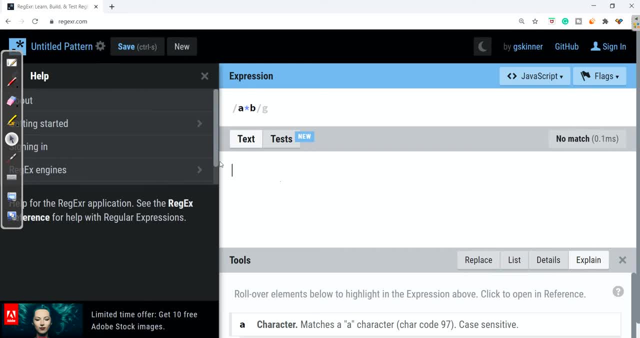 I write star And we will wrap it all. Star means occurrence of last character should be 0 or more. So here, if I write a- b, It is matching. here, If I write a- b, It is also matching. here If I write 2 a b. 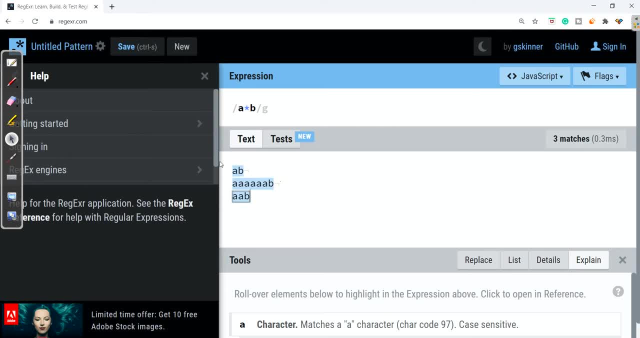 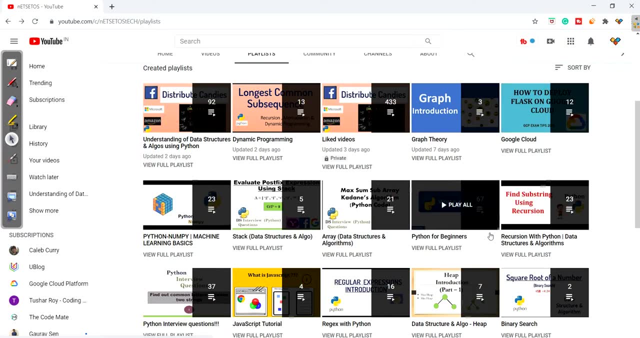 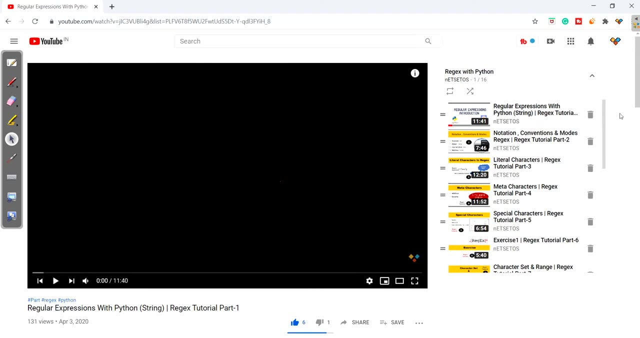 It is matching. So this is all about star and dot. If you want to read this regex in detail, I have made a complete playlist on regex with python. If you click here, You will find a complete package Where you will find literal characters, meta characters, spatial characters, 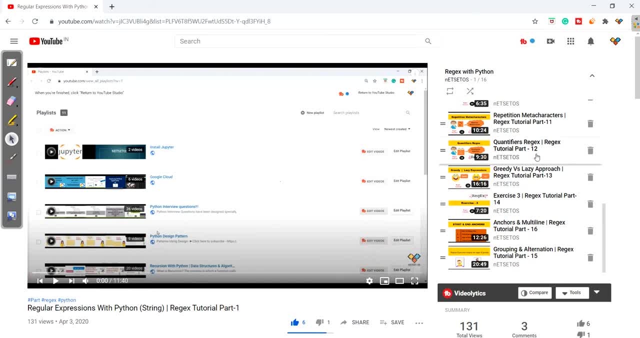 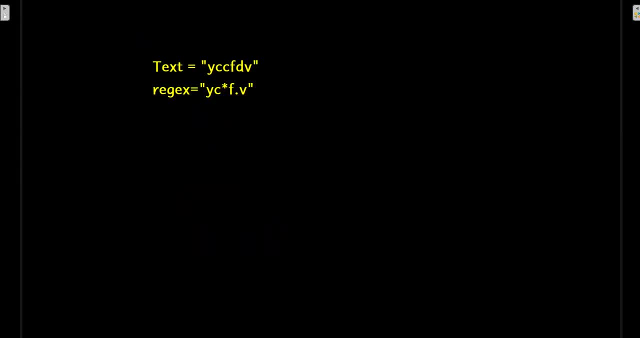 And here I have made a single video also, So you can go for it If you want to read this in detail. Now, coming back to our topic Here, we will take a regex and a text. With the help of this text and regex, 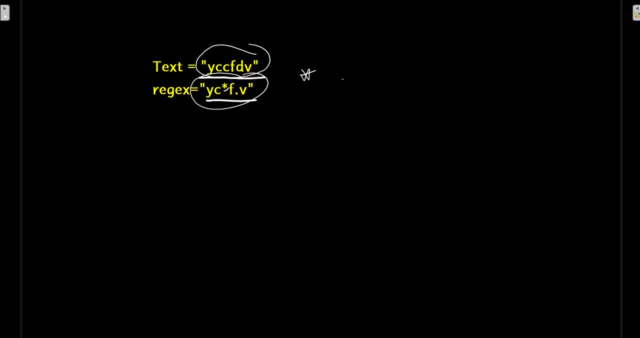 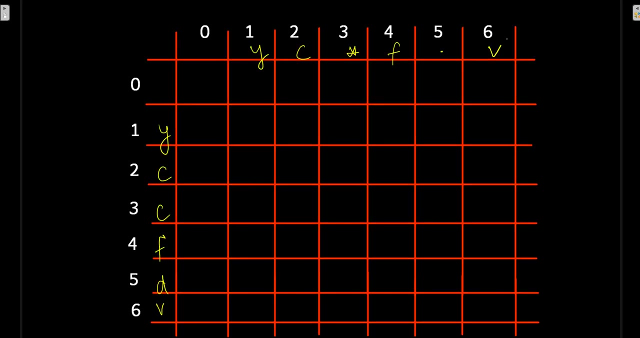 Here in regex pattern I have included star and dot both, And here we will be looking with the help of bottom up solution And we will find out whether this regex pattern is matching our text or not. So here I have taken this 6 cross 6 matrix. 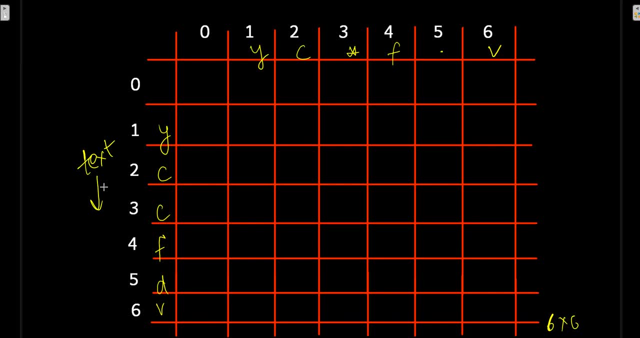 Where? here I have text And on x axis we will put regex pattern. So first of all we will start with 0: 0.. 0: 0 means in regex pattern we don't have anything. An empty string With this text is also an empty string. 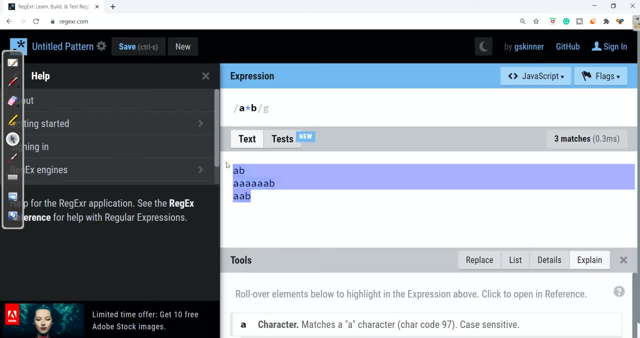 So for 0: 0.. 0: 0 means there is no text over here, Nor any expression over here. So if I want to match an empty string with empty expression, That means it will return true, Because there is nothing to match. 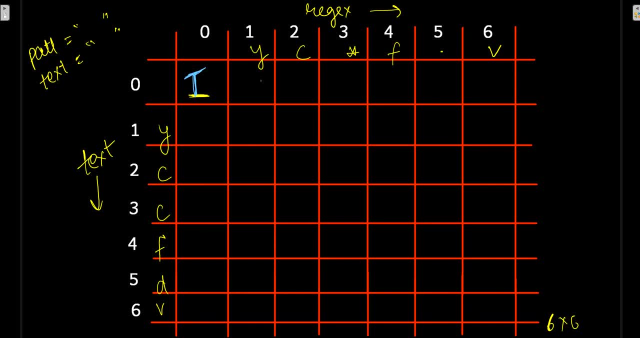 So here I can write true. Now, going towards x axis, Where I have no text, There is no text over here. But coming to regex pattern, we have y. Now imagine you want to match a text Where you don't have any text. 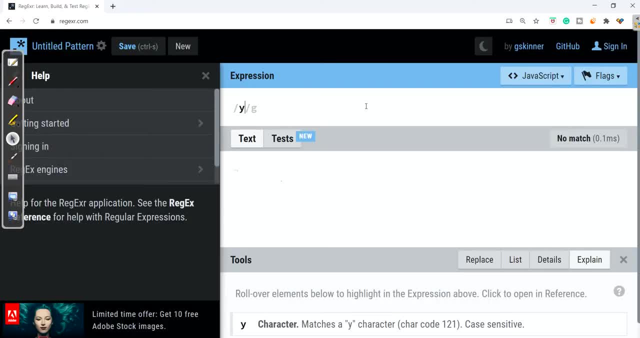 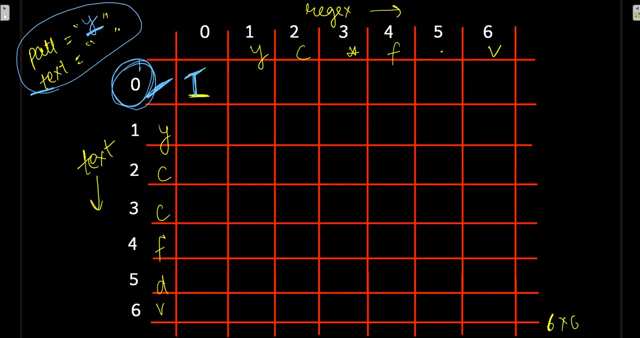 But a pattern. we have y Here. I have put an expression, A pattern, over here, y, But I don't have any text to match with it, So it won't be returning anything. It will be returning false. Now you don't have any pattern. 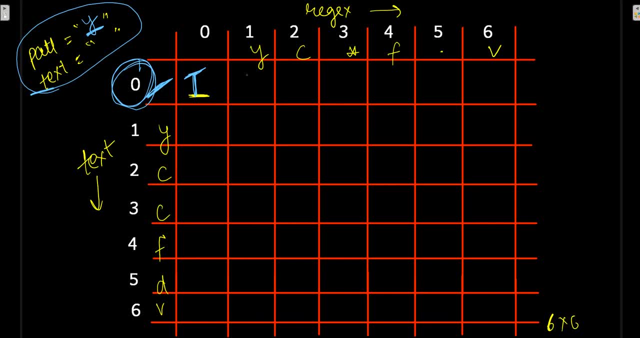 With which it can match the text. So here it will return false. If we think vice versa, Here we have y, But we don't have any pattern to match with our string. That is also the same case If we don't have any pattern. 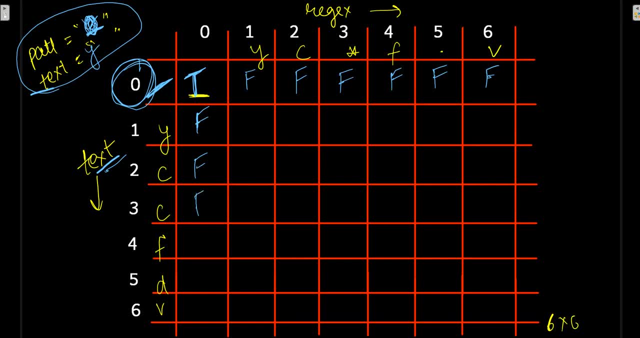 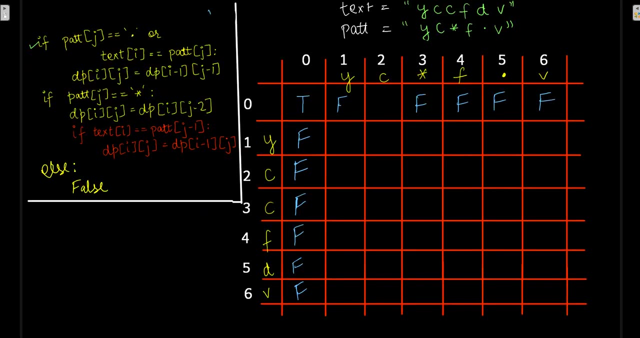 It will return false, Right. So with this we have filled first part of our column and row. Now we will be filling the inner part of our column, Matrix, Where we will take the help of this algorithm. Let's make this false. 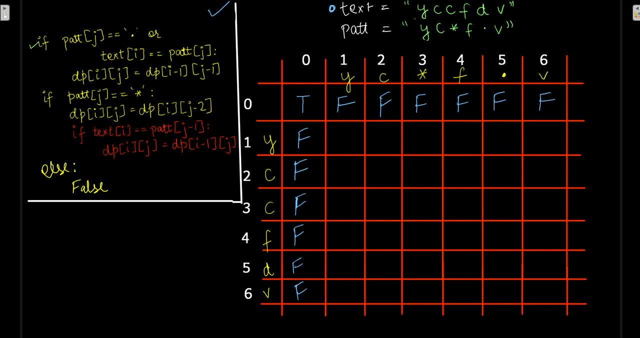 And we have a same text and a pattern. So this is i and this is j. Let's understand our algorithm first Here. it says: If you have text and pattern match with each other, That means we have text a And a pattern a. 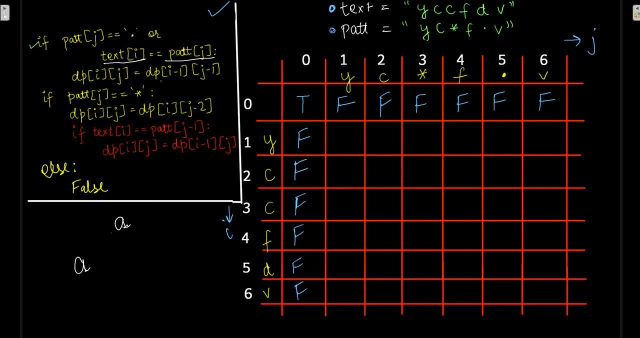 When it matches with each other, It will look for its diagonal form. Let's take an example. If I have in pattern a And in text it's ya, So as to match expression a with our text, A will match with each other. 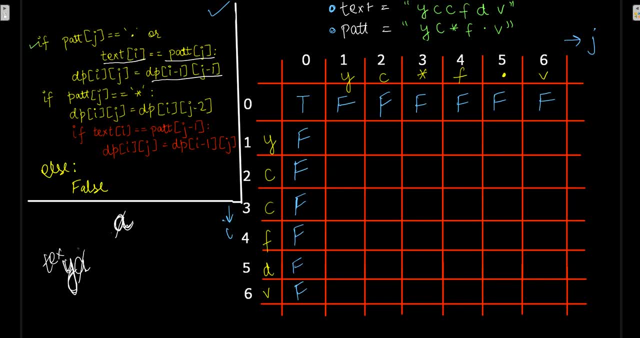 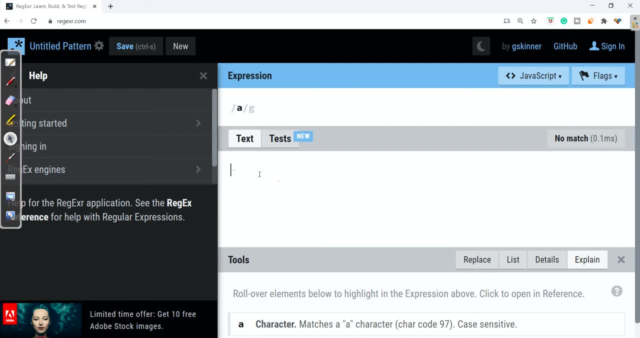 But what about y? Y won't be matching with it. Let's see it on the side Here: in the expression I have a And in text I have y. So what it will do, It will match our expression a part. The last part will match with each other. 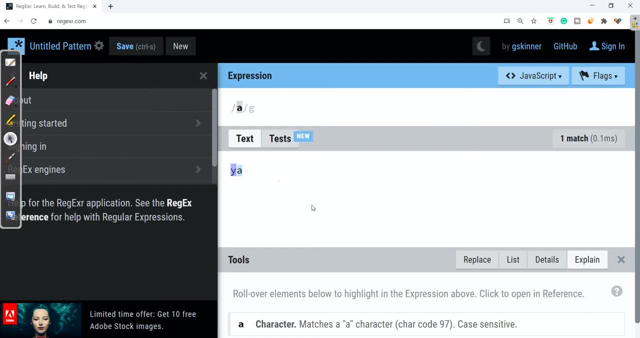 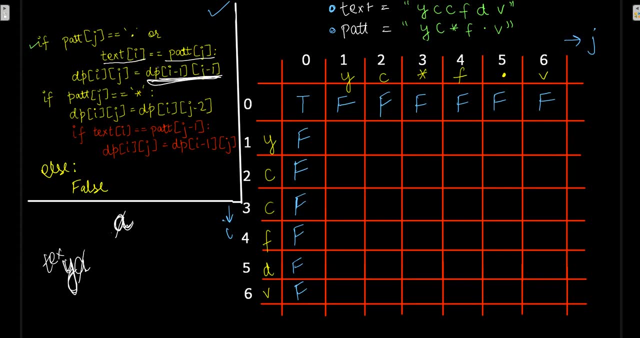 But this y won't be matching with our expression, So that's why it will look for its diagonal form. So it will look for its before part, Whether it is also matching with our text or not. Similarly, for star pattern, It will look for two column before. 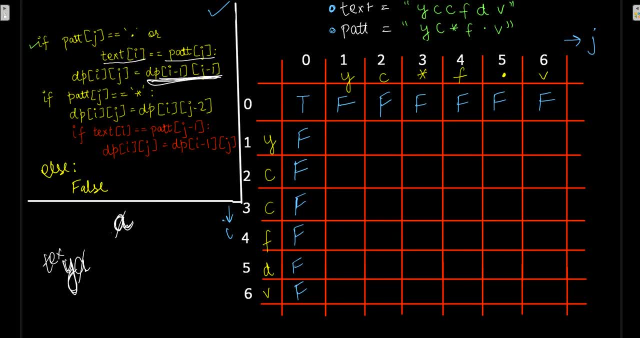 j minus 2.. How I will tell you. Let's say, if I have in my pattern c a star b And here in my text It has been given c b. Now coming to text, and pattern B will match with each other. 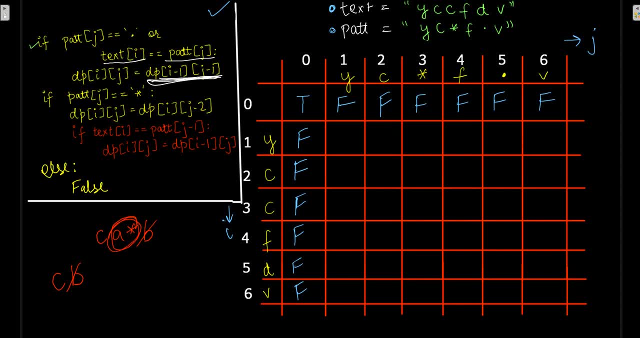 Now coming to star. Star is for occurrence, For its last character, If it is zero or more. So here there are two characters. If it is not there, It will look for directly. c, Two columns before. Let's understand this with the flow. 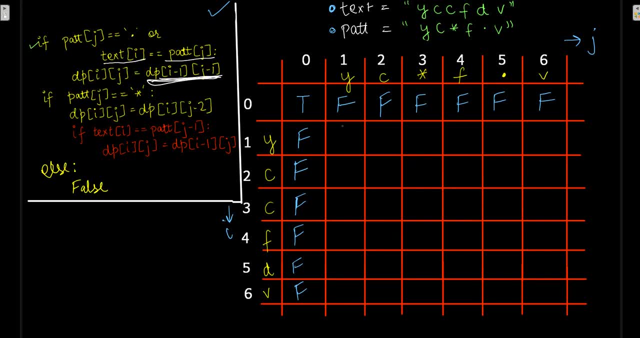 So here we will fill out this. First of all. it says on one part: We have my pattern, Here I will write pattern And this is text. We will write on both side simultaneously. So for pattern it is y And for text it is y only. 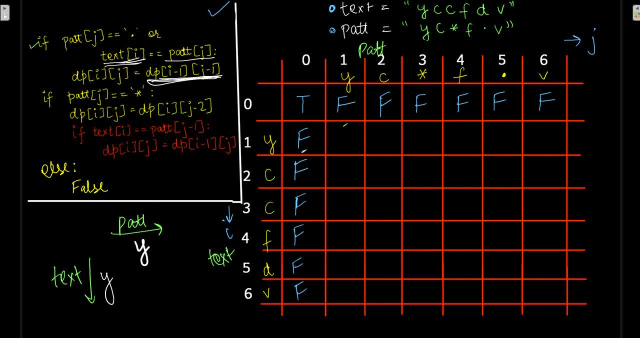 So it will look for text i. Text i, y and y are matching with each other. Yes, they are matching. So it will go within And it will look for its diagonal part. If it is true, Here also it will return true. 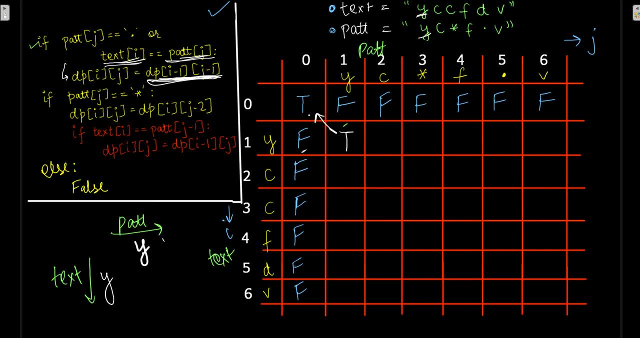 Let's take more Here. in pattern we have y, c, Whereas in text we have only y. Will y c be able to match text y? No, So here it will return false. Then pattern will be incremented To star y c, star. 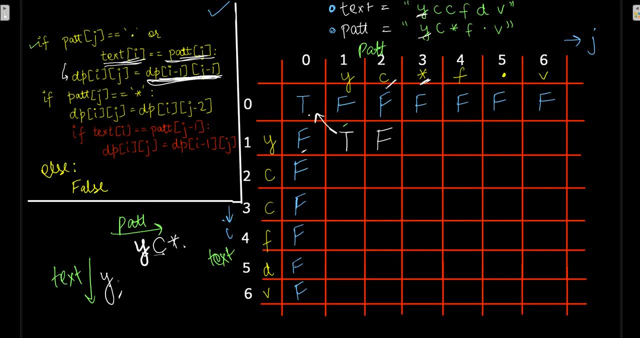 Whether y c star matches with y. We will look into algorithm afterwards. Just try to understand, with its star symbol, The occurrence of c. If it is 0 also, Then also it will match with y. So here, y c star, c star, if it is not there. 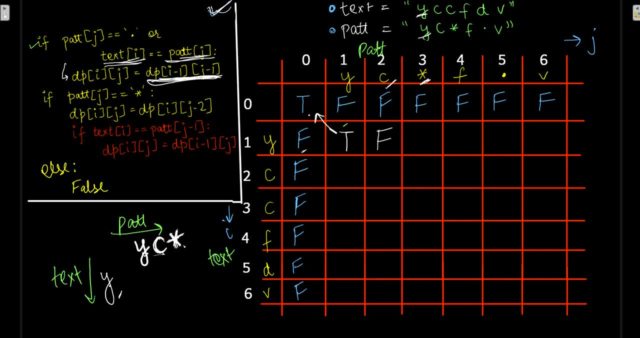 It will match with each other. Now if we look to our algorithm, It says: if we have star over here, Then it will go 2 columns before With j minus 2. And here it is returning true. So here I will write true. 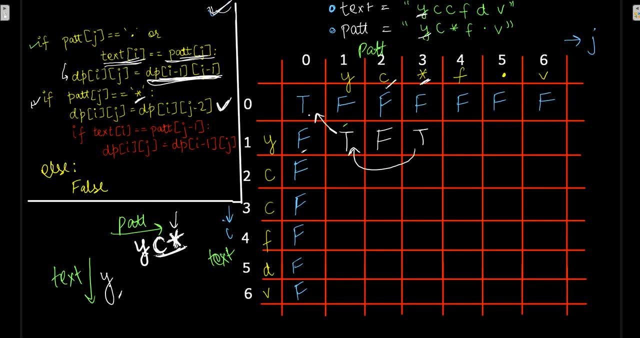 Because it looks for occurrences of c. If it is there And the occurrence of c Can be 0 or more, And in this case it was 0.. Now we will look for f y c star f will be matching with our text y. 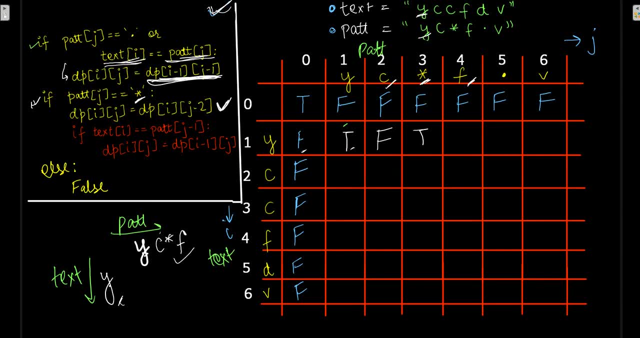 No, It simply looks. It will not match with each other, So here it will return false. Then for dot: Here I will put dot. Whether dot matches with y? No, Because pattern is increasing, But text is just y, So it won't be matching. 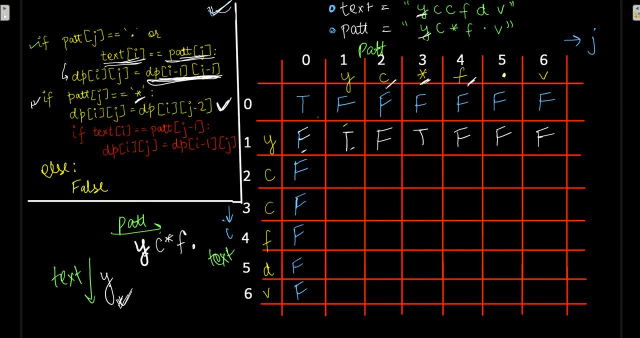 It will return false. Now we will turn Up with algorithm. also We will understand with the help of Algorithm from now onwards. Here we have In pattern just y, And in text We have y, c, So, c and y. 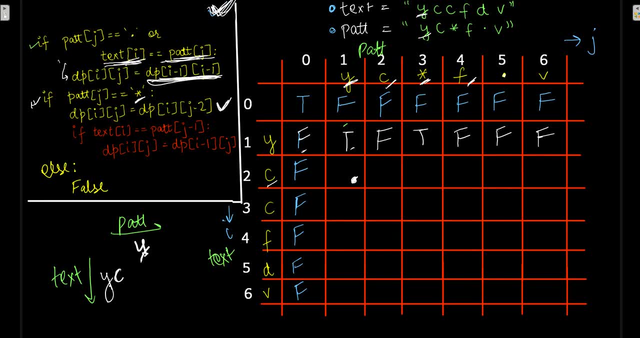 Is matching with each other. No, So it will look for Other if. condition Is it having star? No, So it will go to else part And will return false. Now It will go here And will look for y c. 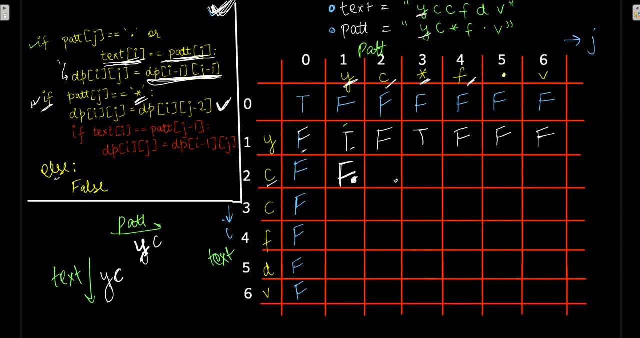 In the pattern As well as in the text. We have y c, So in c C Is matching with each other. Here It matches with each other. For text type, Pattern j, It Is equal to each other. 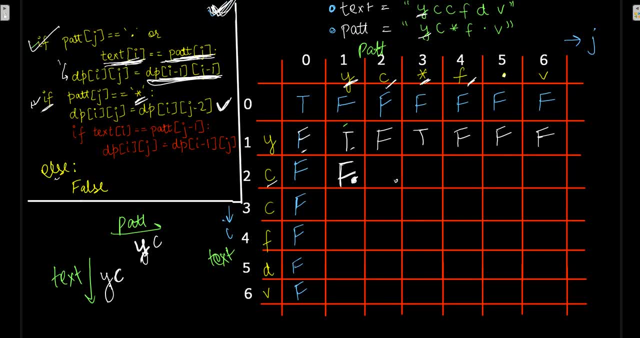 As both have c. So it says To go Diagonally And will look for y c. So it says To go Diagonally And will look for y c. So it says To go Diagonally. 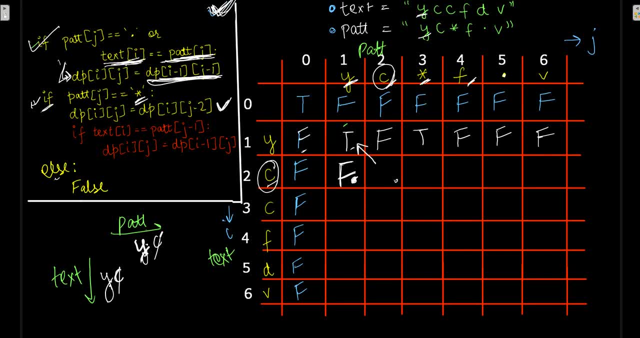 And will look for y, Where the y is Equal to each other, Which we have Already seen And returned True. So here also It will return True. Now in pattern We have y, c Star. 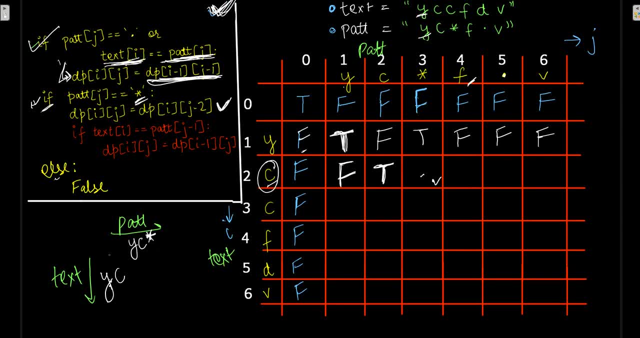 Now For the star And c. Here It will go to Pattern. j Is equal to Star Because Pattern has Star. So it will go into If condition And says To look for Two columns. 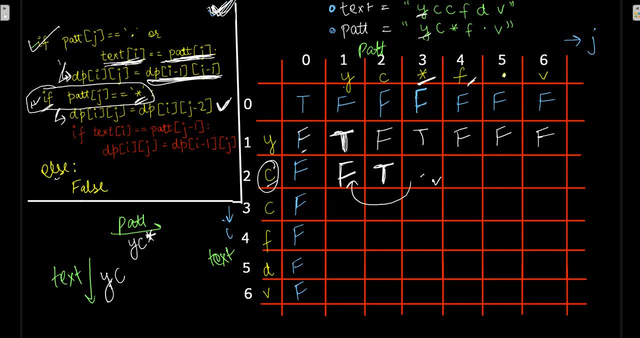 Before, But here It is returning False, So it will go Into if condition Will look for Where the Pattern J minus One, J minus One is C, So c Is equal to Text. i. 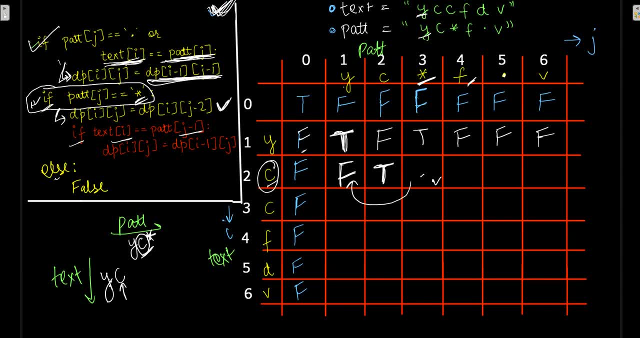 Why is it Going for J minus One and i J minus One For its One occurrence? If This c Is matching With This c, It will Go Above And will Copy This. 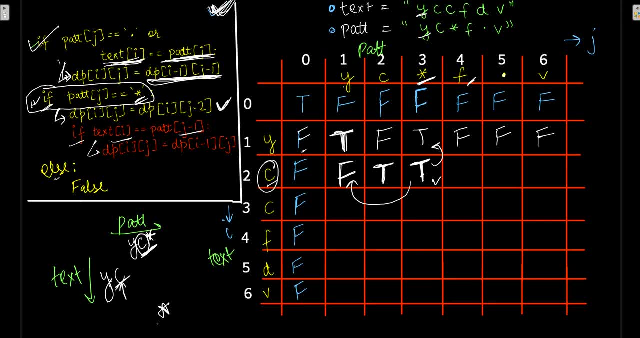 True. So for Star Case We have Two condition: If Occurrence Of Last Character Is Zero, It will Go To Columns Before And Look For The Row. 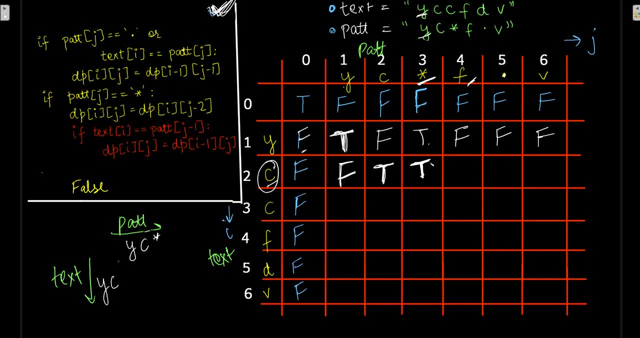 Above It, As It Was True. So Here We Got. Now For This Part We Have F. F Is Looking For C. Whether F Matches, Whether 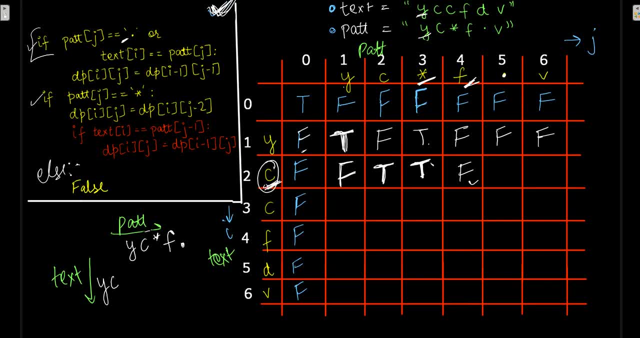 Dot. Yes, We Have In First If Condition Dot. So Here It Will Look For A Column In Diagonal. So In Diagonal We Have False. 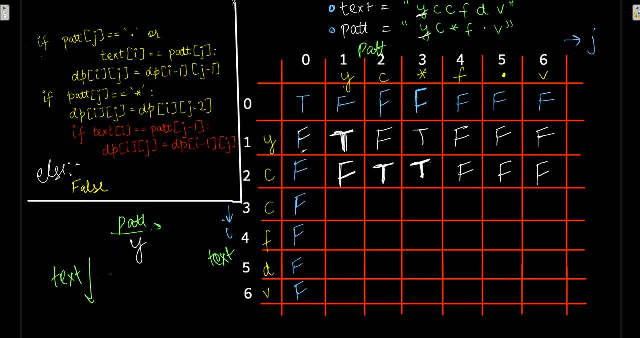 So It Will Have C. Let's Write The Complete Text Y, C, C. So We Have To Match C With Y First. We Will Check. 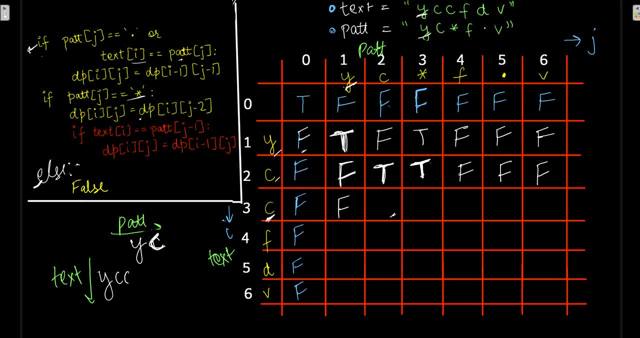 In This F Condition Is It Matching With C? So It Will Go To. If Condition Text I Is Matching With Pattern J, That Means We: 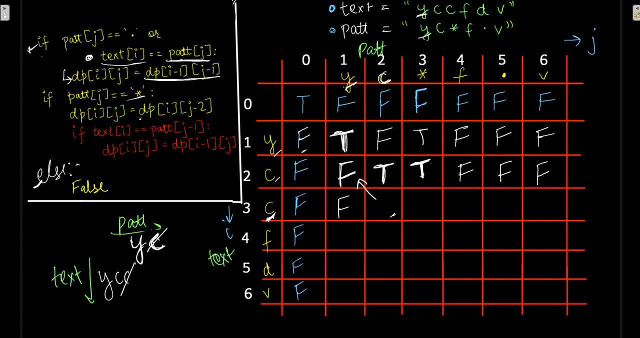 Have C In Both Cases, So It Will Go Into Match Y, C, Two Characters, So Here It Will Return. False Now Here In Pattern We. 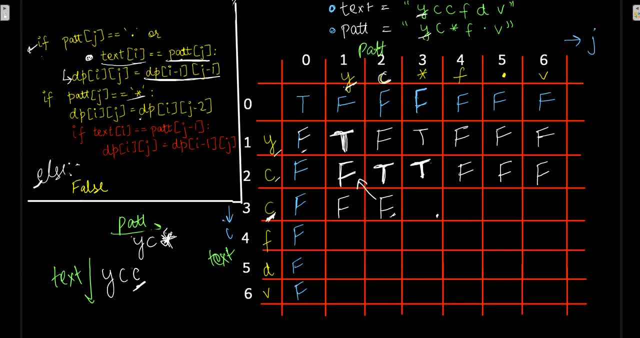 Have Y C Star, Whereas In Text We Have Y C C Now In Pattern. It Will Go Inside If Condition And Here It Will Go. 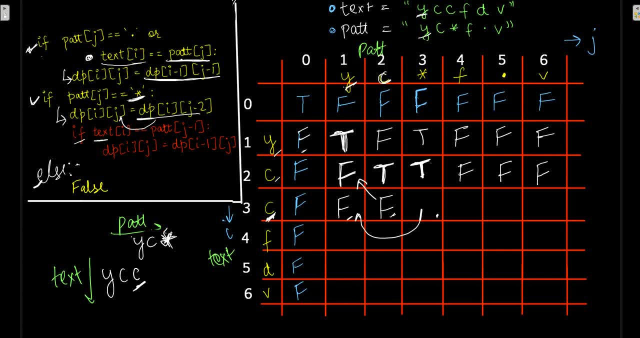 And Check Two Columns Before It. So Here It Says: False As It Is Returning, False Of It Which Is Returning True. So Here We Will. 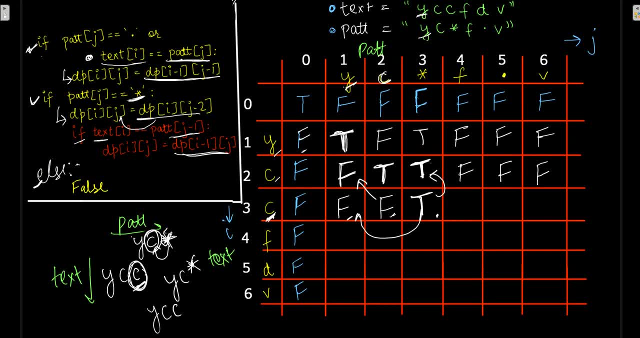 Have True. Now Try To Think It Otherwise. Here We Have Y C Star, And In Text We Have Y C Star F, Whereas In Text 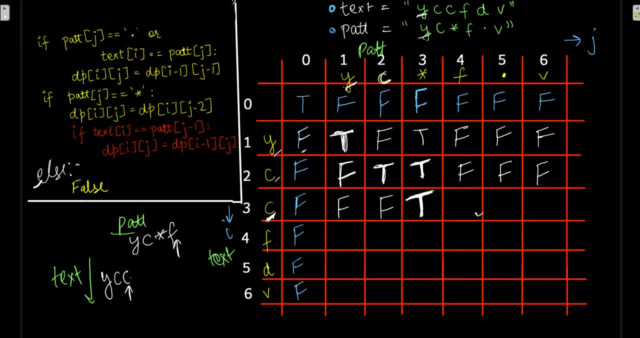 We Have Y C C, So We Will Look For F And C Whether They Are Matching With Each Other. No, Neither We Have Y C. 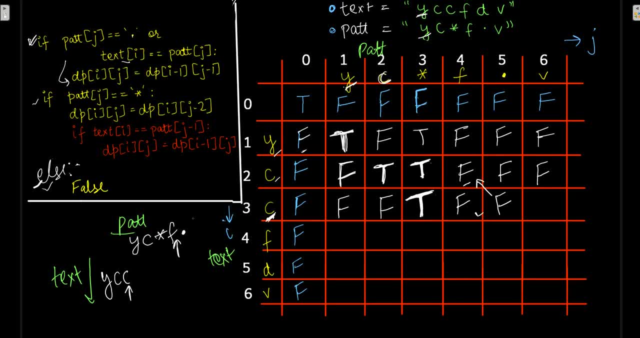 C F, Whereas In Text We Have Y C C F. No, Neither It Is A Star, So It Will Go To Else Part And Return. 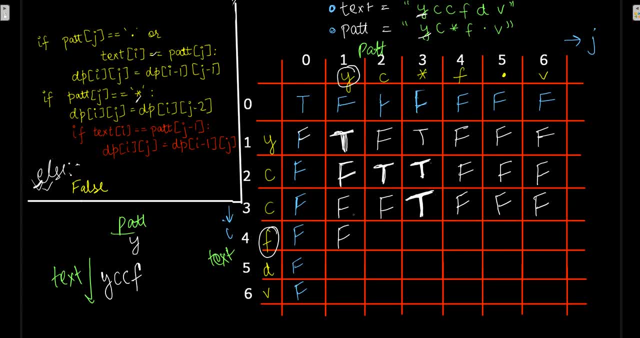 False, So Here It Will Return. False Now We Have In Pattern Y C. Is C Matching With F? No, It Won't Be Going Any. 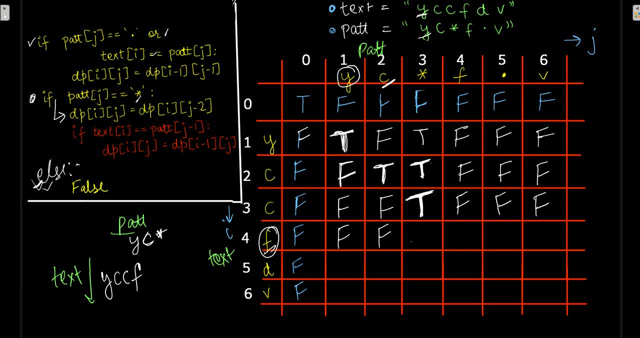 Of The If Condition, So Before It, Where It Says False. So It Will Check The Other If Condition Also Whether The Element Before It Which 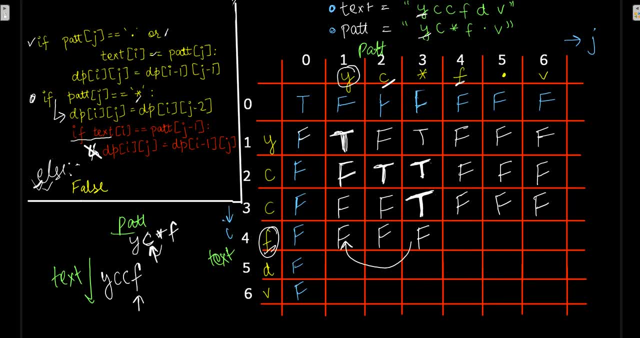 Is C Is Equal To F. No, So It Will Go Inside If Condition And Look For First Diagonal. So Diagonal Is T So Here. 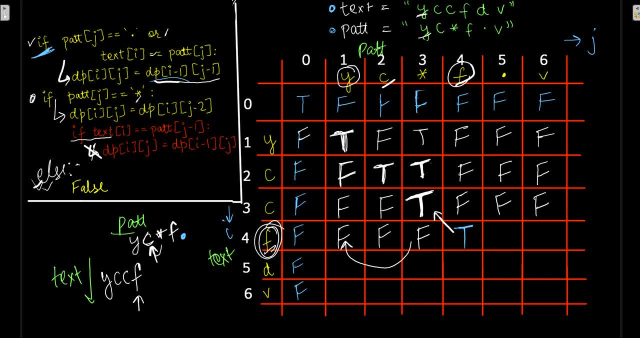 We Will Get True. Then For Dot Y C, Star F Dot, It Will Return False. Now For This Part, We Have D Y C C. 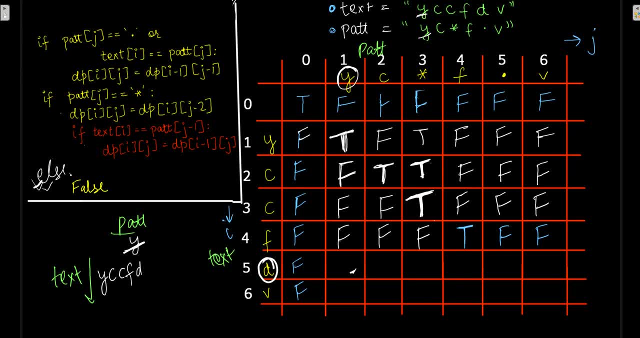 F, D. There Is In Pattern We Have Just Y, So We Will Be Looking For Star Star. It Will Go To This If Condition And 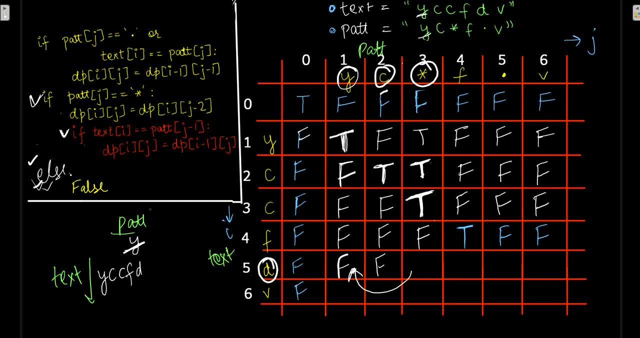 Will Check Two Columns Ahead. It Is Returning False, So It Will Go To Other. If, Whether The No So Here It Will Return False, Then 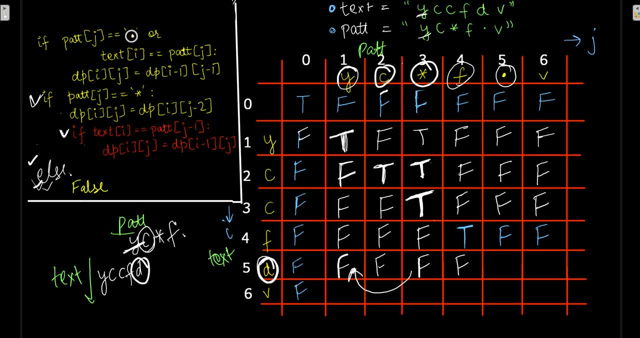 For Dot. Is Dot Matching With D? No, But Here We Have Dot, So Here It Will Go Inside This F Condition. Then For The Last. 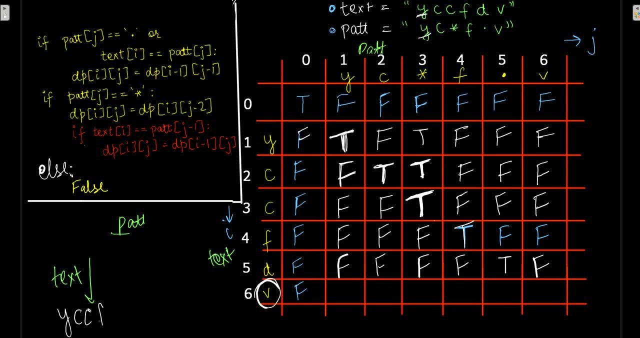 Column We Have V Over Here. Let's Write The Complete Text Y, C, C, F, D, V And In Pattern We Have Y, So For: 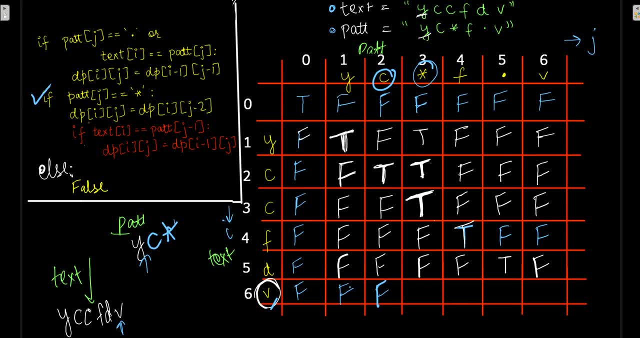 Star. So For Star It Will Go To F Condition And Will Look For Two Columns Before Where It Is Returning False. So It Will Go. 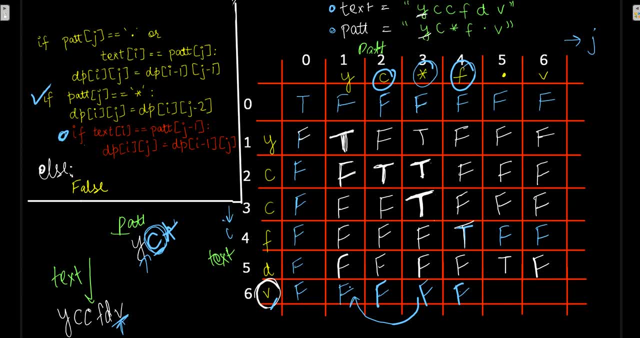 Inside F Condition, Then For Dot Dot, If Condition And Will Have Its Diagonal Part, Which Is False, Then For V Is V Matching With. 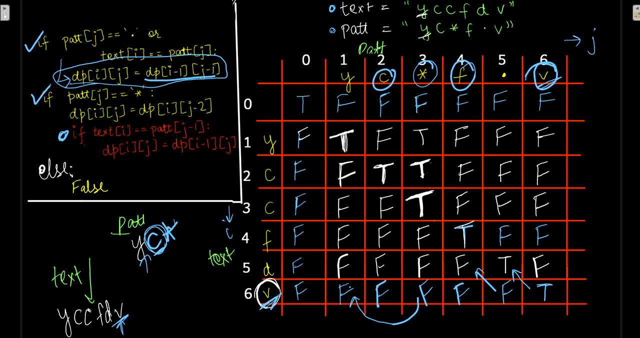 V. Yes, It Is Matching. So It Says: This Pattern Is Matching Our Text. So Hope You Got The Concept. Star For Star. We Have To. 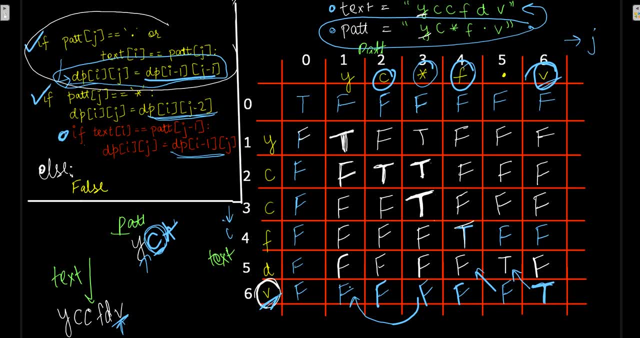 Look For Two Columns Before, And Then We Have To Write Python False. As Simple As That. Now Coming To Writing Python, It Will Be Same. 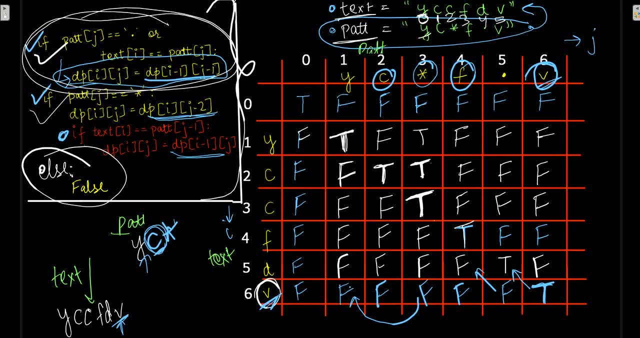 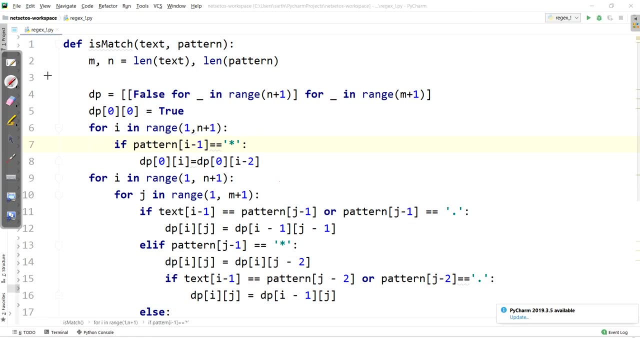 As This Algorithm, But, As In Python, We Will Start From Zero, So We Will Reduce It By Minus One, As Like This Here: First: 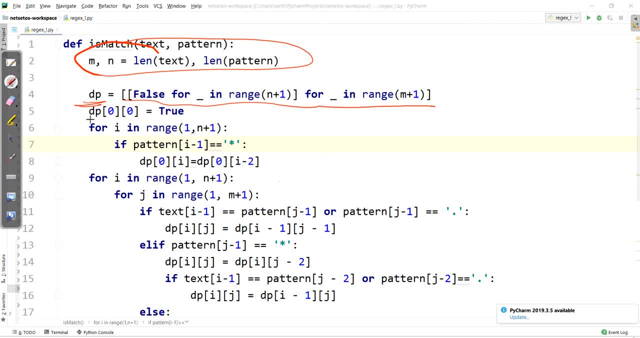 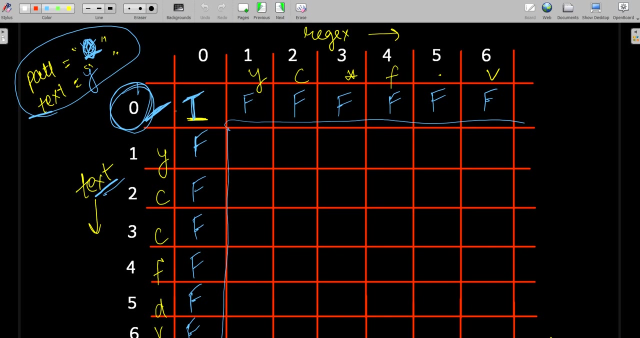 Of All, I Took M And N, Then I Have Made A D P Where I Will Come, Which We Have Written Over There And With 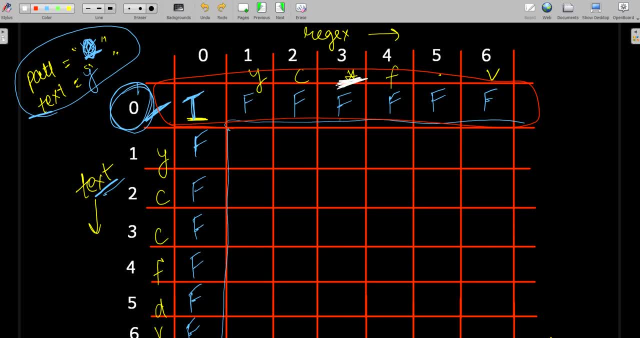 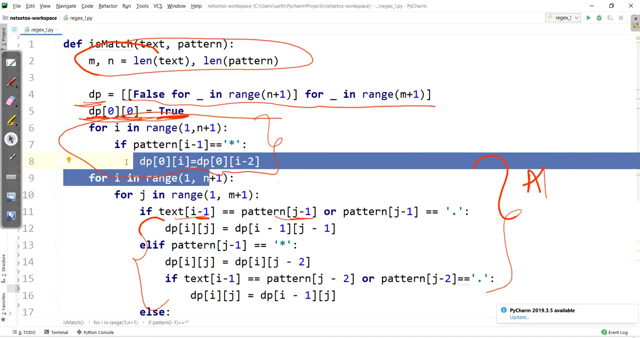 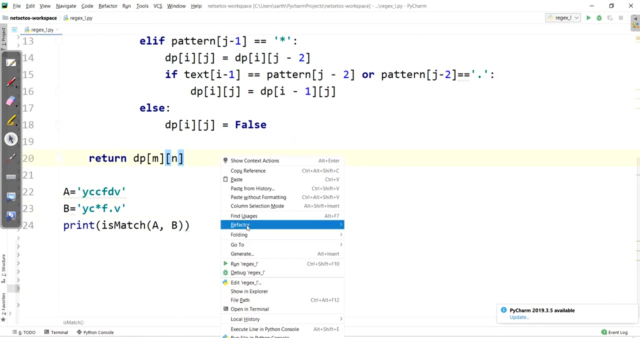 This. We Have Also Written This. When We Were Defining First Row As In, We Had Star Over Here. Here I Took The Same Input. 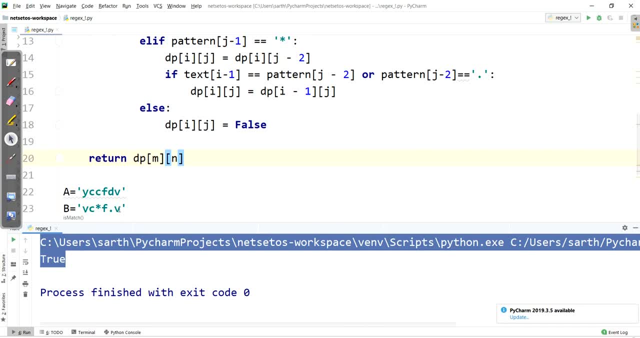 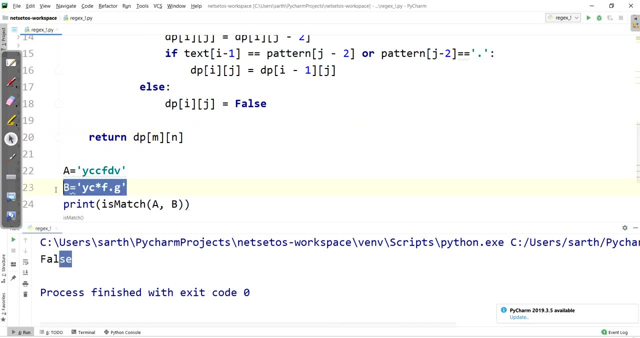 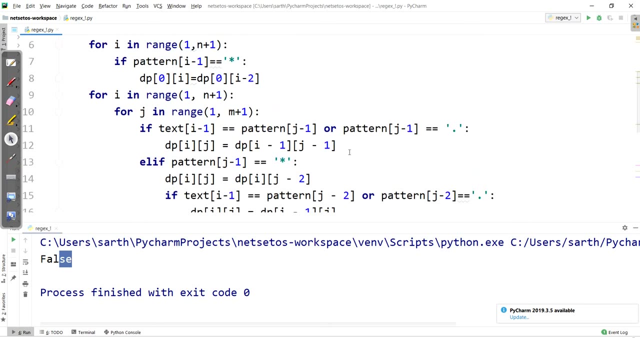 Let's Run The Program. And Here We Got True Now Instead Of We. If I Write G And Run The Program, I Got False This. 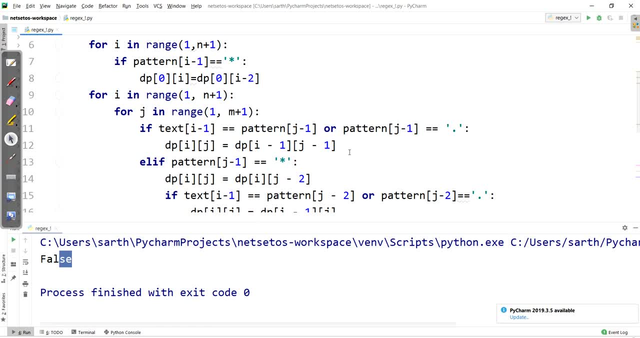 Concept Or Any Point. You Are Missing Somewhere, You Can Let Me Know In The Comment Section Below. I Will Explain It In My Next.